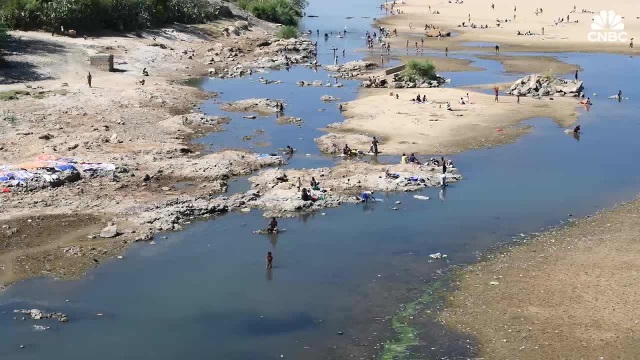 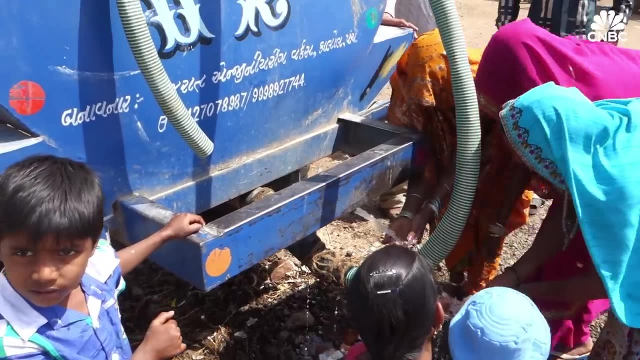 this may be its most valuable investment, yet The United Nations estimated that by 2025, 1.8 billion people will be living with absolute water scarcity. If you don't have water for people, animals, plant, communities, as a nation. 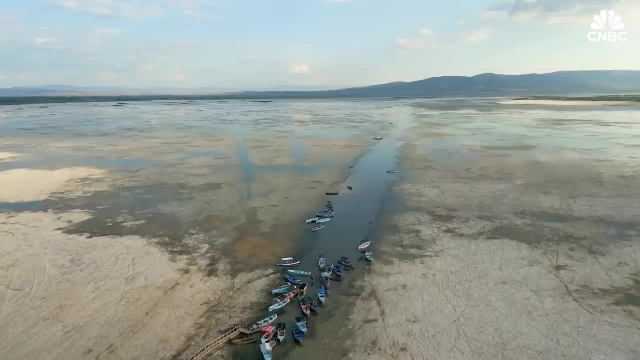 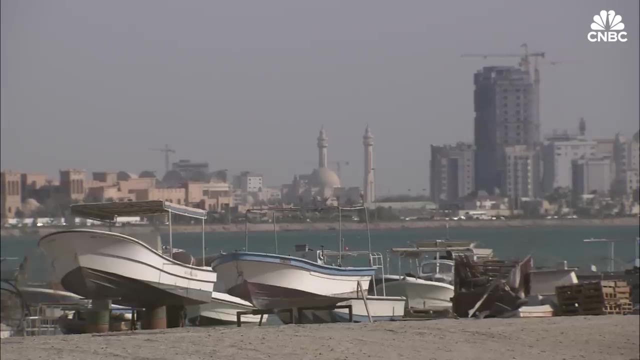 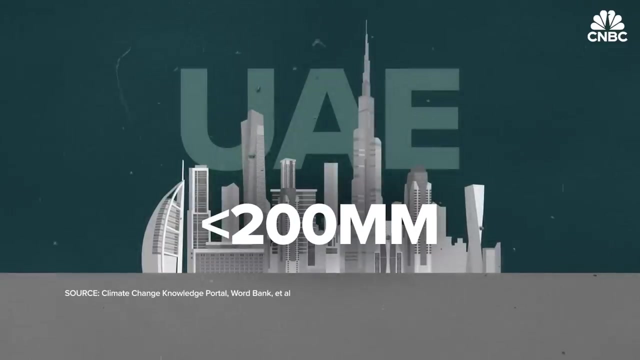 you will really struggle, especially in desert countries. Increasingly, lack of water due to climate change is resulting in less secure water, And the Middle East is home to 12 of the 17 world's most water-stressed countries. The UAE receives less than 200 millimeters of rainfall each year. To put that into context, 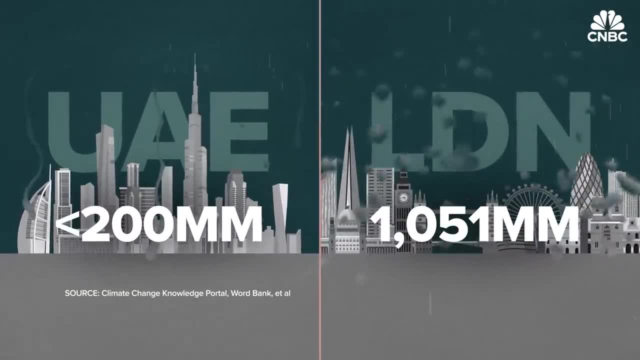 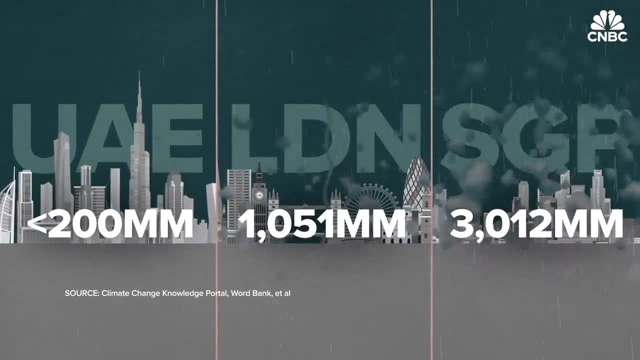 London soaked up an average of 1,051 millimeters of rain in 2022.. While Singapore drenched in a whopping 3,012 millimeters during the same year. So, as one can imagine, ensuring enough water for the UAE's population is a real challenge. 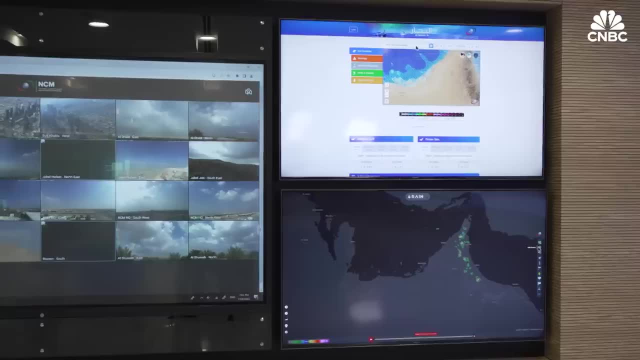 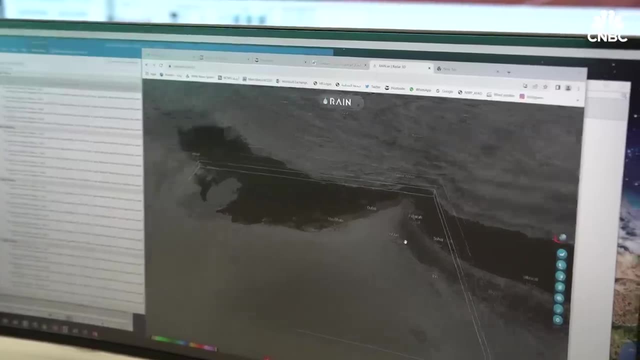 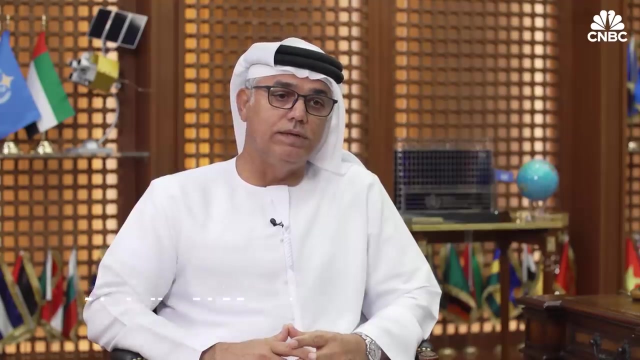 To continue to support its increasing development and growing population. the UAE government invested more than 20 million dollars in research to start a process called cloud seeding. Cloud seeding enhances the rain in the cloud. The main objective of that is to increase the storage of the groundwater. It was a direct order from His Highness, Sheikh Mansour. When did this start? It was late 2000 and early 2001.. We were partner with the National Atmospheric Research in the United States. The entire Gulf region could face a 50 percent reduction in water availability per capita by 2050. 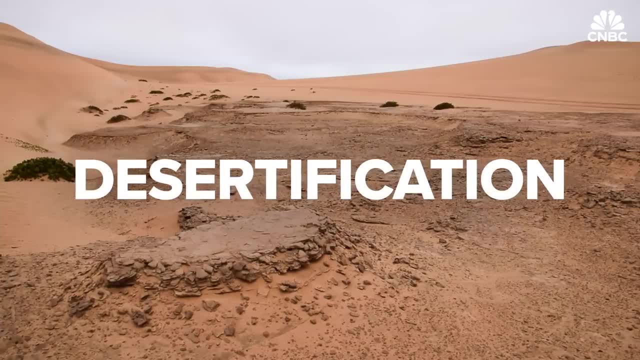 The UAE has tried to combat desertification, which is a land that is no longer productive because it can't support plant agriculture Existing expert Hariri ran�, who came out for a talk, in fact, earlier this year to explore the project Transpicting sand in the ground. the UAE claims soil resources are lipid splashes for plant environment storage. 天aling requires water desertification and there is no suitablehelm to support the rework on lamenting by a general problem. suddling might not organize those areas because some of whom say that global forest줘herty the responsibility of over-examination and include the government's policies. 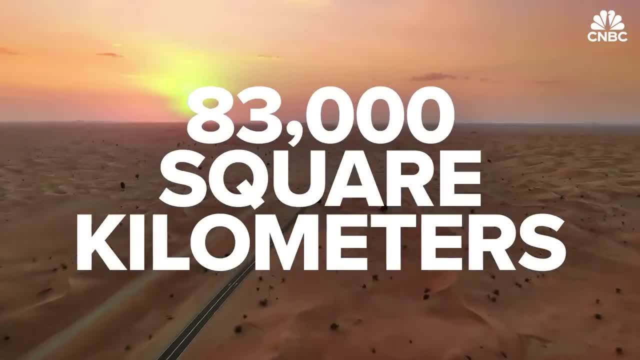 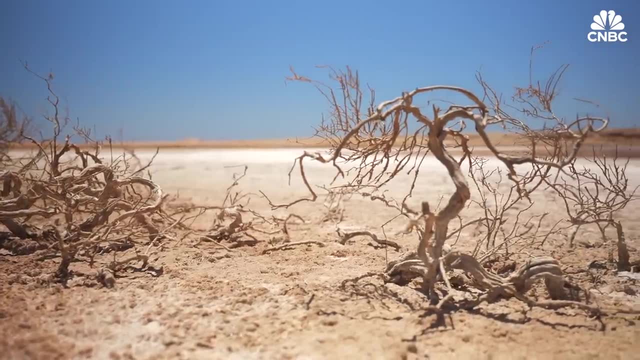 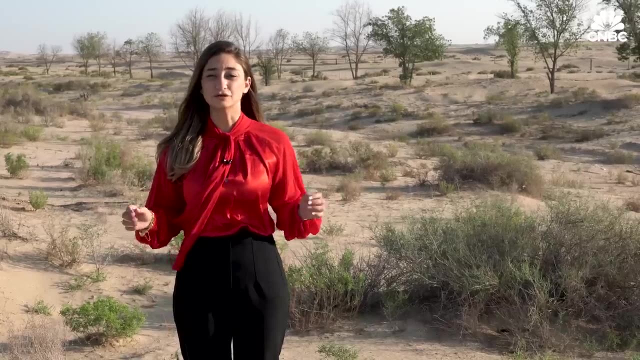 growth. The Emirates spans over 83,000 square kilometers and around 80% is desert. It's estimated that 75% of a planet's land is already degraded. These lands have become deserts or are uninhabitable. About 12 million hectares of land is lost around the world each year as a direct consequence of. 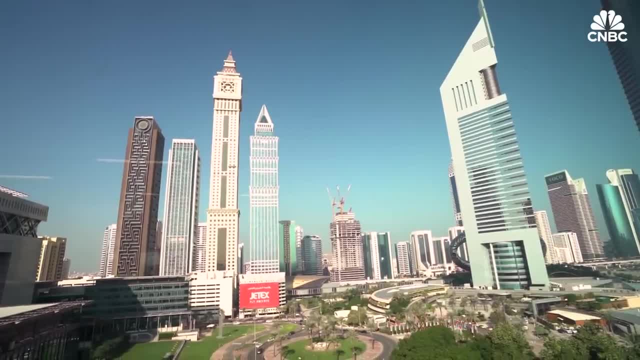 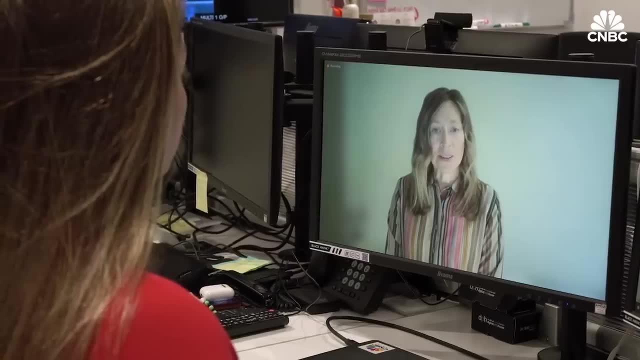 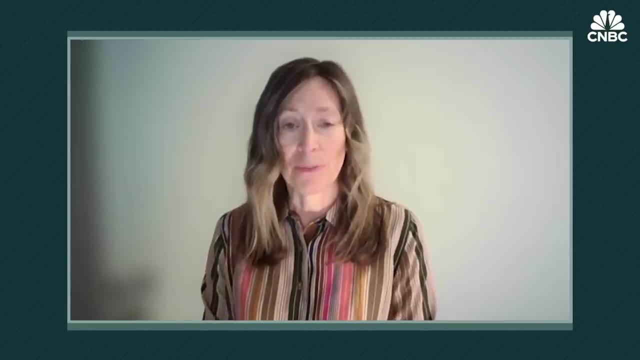 drought and desertification. The World Bank estimates the Emirates has lost almost 33,000 hectares of land from 2002 to 2018.. So the decrease in arable land is primarily due to land degradation. So this impacts over 3 billion people and people that live in desert and dry. 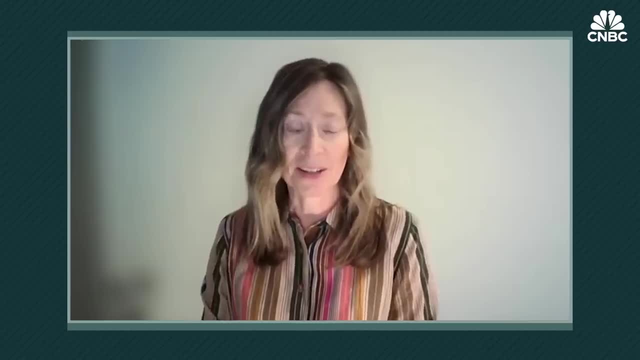 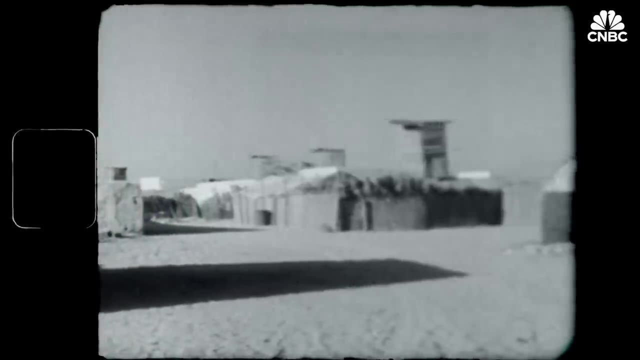 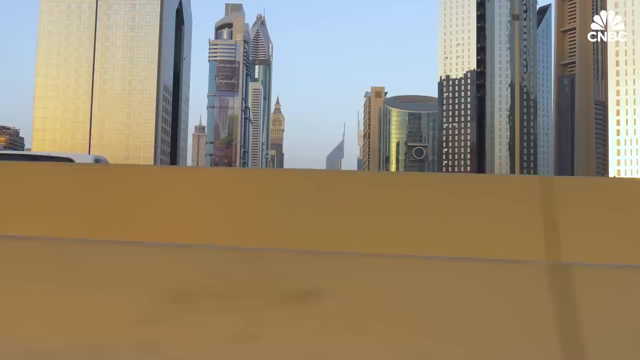 land ecosystems that cover nearly half of the globe are particularly vulnerable to the loss of arable land and land degradation, But in the last 50 years, what was once a large desert and a tranquil fishing port has evolved into an urban metropolis. Long before skyscrapers and bustling cities, the UAE had a history of planting trees. 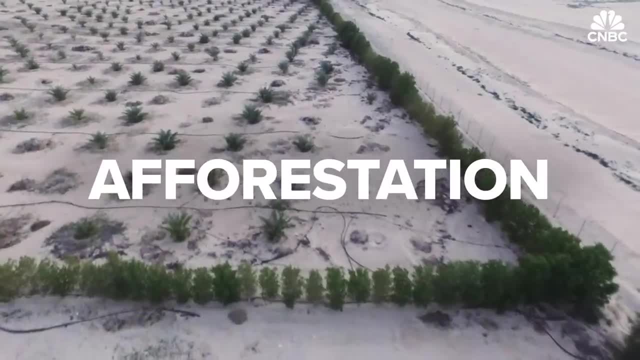 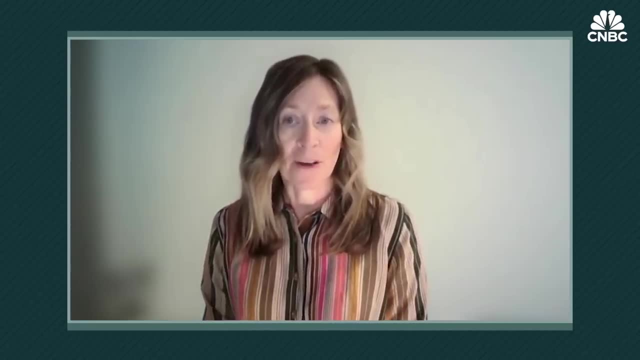 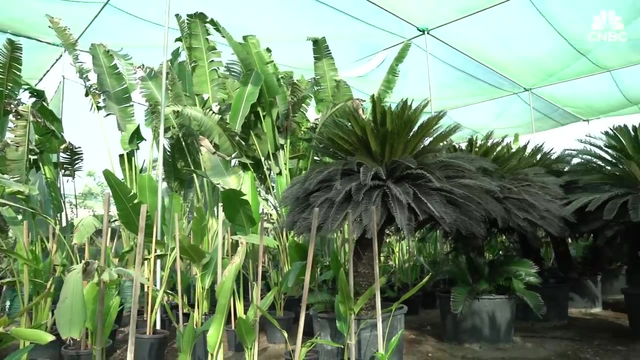 in areas that lacked them, a process called afforestation. What we're seeing across the world, especially some of the countries that have significant desert systems, is efforts to green the desert, which means bringing in trees, other plant communities to increase as the initiatives. 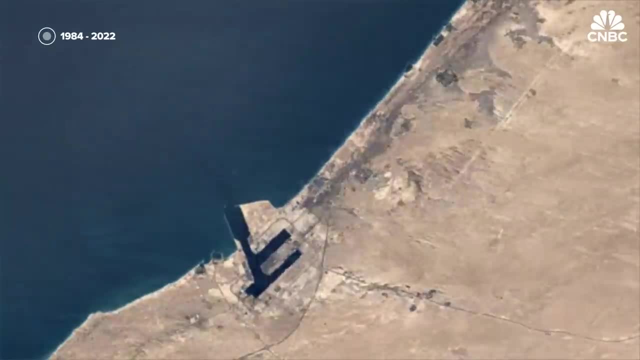 say the greenness of the deserts. Take a look at these satellite images of the UAE in the 19th century. The UAE was the first country to have a desert system. The UAE was the first country to have a desert system. The UAE was the first country to have a desert system. The 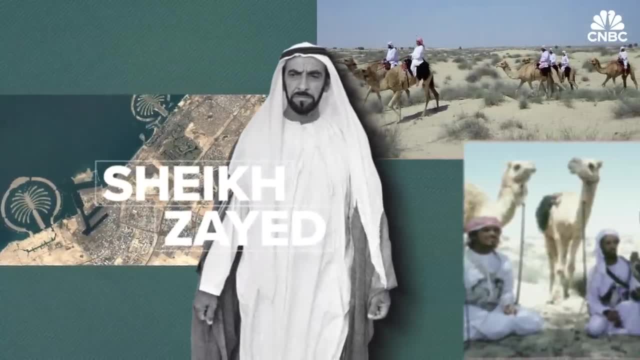 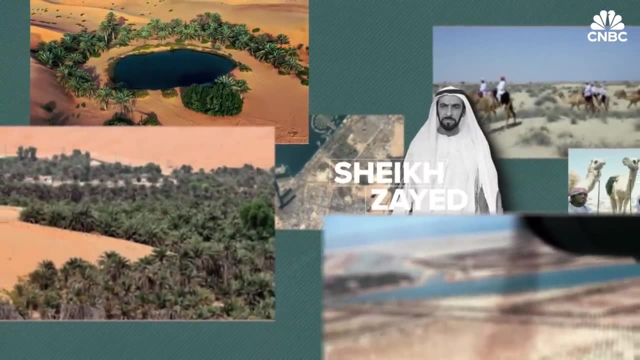 country's late president sought to provide permanent homes for nomadic Bedouins in the parched desert. His dreams set the stage for a nation's ambitious end of war, and their leaders knew that trees could help with the fight against desertification. About two decades ago, the 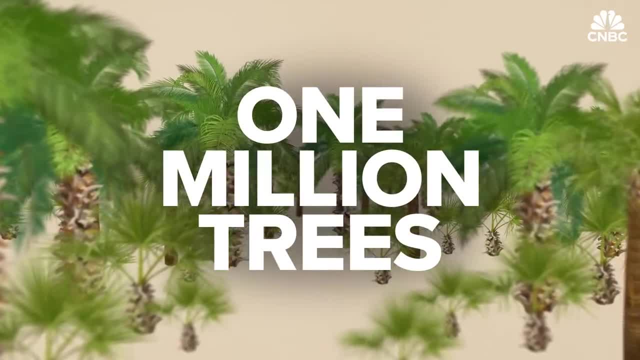 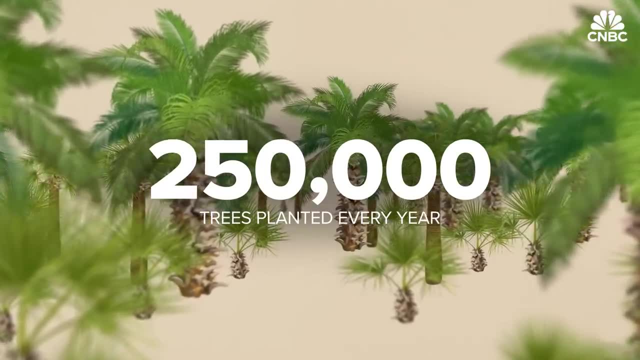 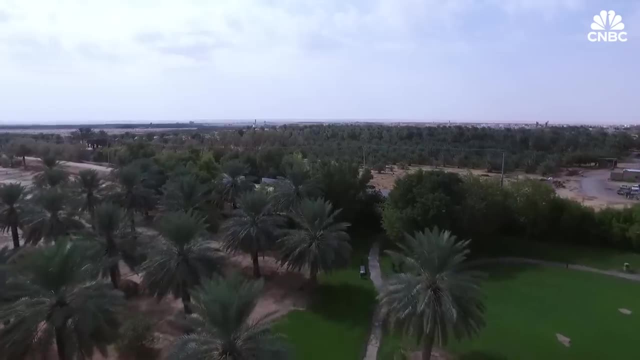 One Million Trees initiative was announced by the ruler of Dubai. The plan was to plant 250,000 trees every year in collaboration with the Dubai Police Academy. It wasn't long before rows of olives, palms and the Brazilian gaffes- the national tree of the UEE, painted the once. 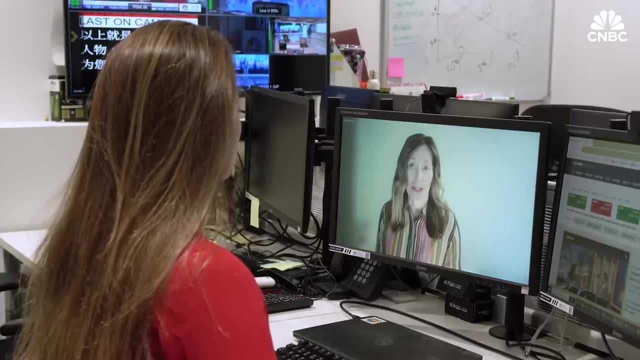 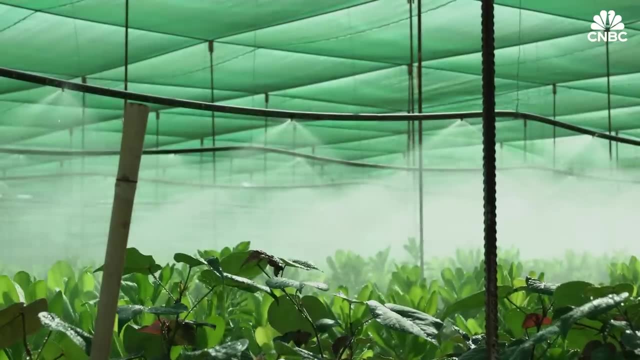 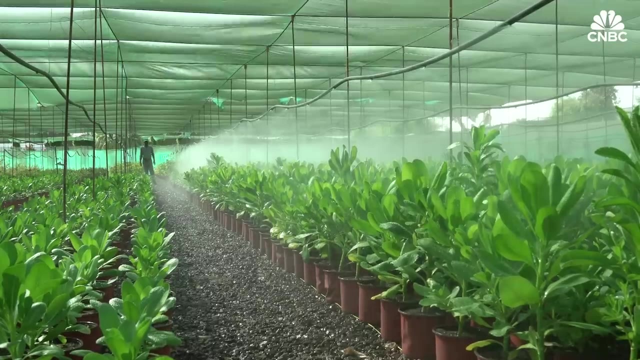 empty land with life. When you are planting some of those trees, you can dig different holes to capture water and engineer the landscape, so those trees that you're bringing in will be able to survive, And so that's critically important is that it's not only the types of trees that you're 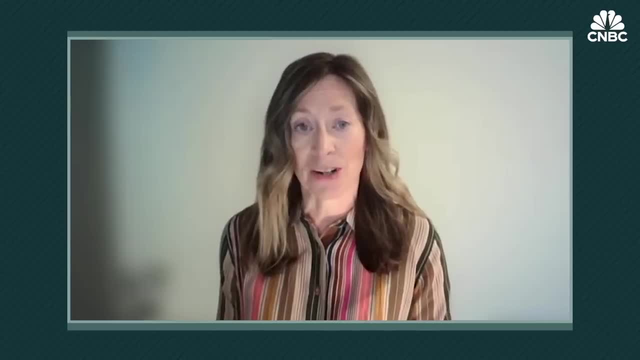 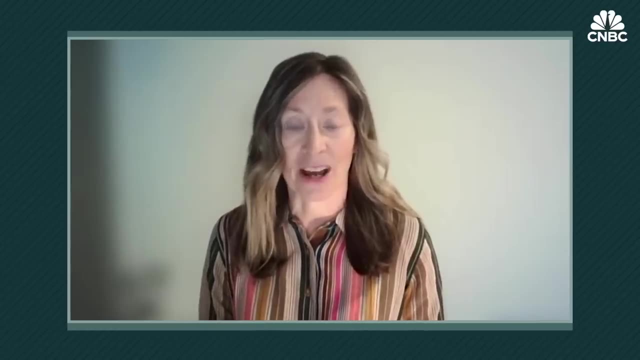 bringing in, or the types of plants you're bringing in for these afforestation projects, but also how you engineer the landscape to be able to receive those plants and that they are able to survive. A tree nursery for the One Million Trees Initiative was created, spanning more than 130,000 square meters. but challenges loomed large over green dreams. Behold Mall of the World, a mega shopping center project. It was said that Dubai, Holding the investment vehicle of the Emirates ruler, would require $6.8 billion to build that. 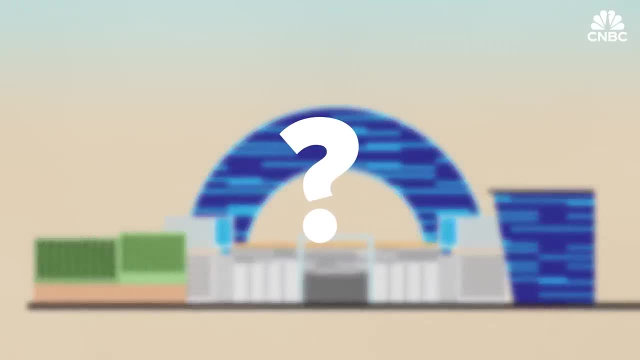 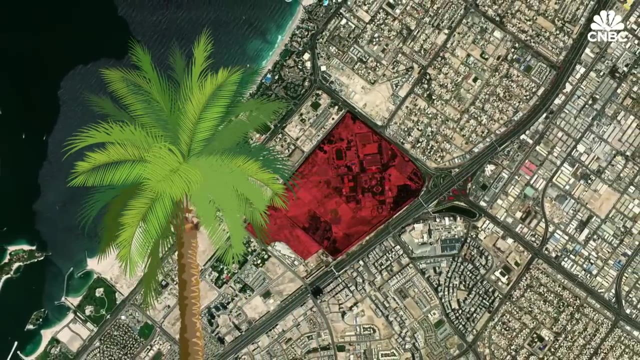 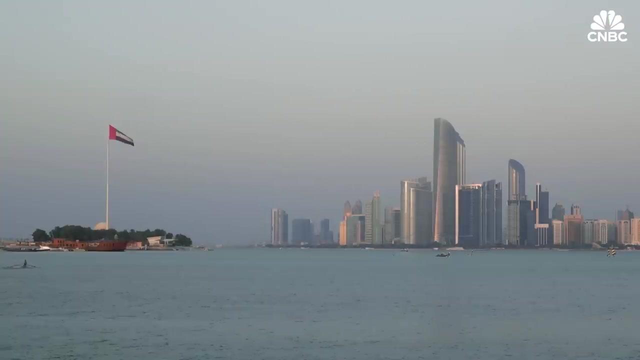 entertainment district. Could you guess where they wanted to build this mega project? None other than the very land the tree nursery once thrived. And just like that, the project fell through and thousands of trees withered away and died. But in January 2015,, the UEE cabinet approved the UEE Green Agenda for 2030, aimed at building a 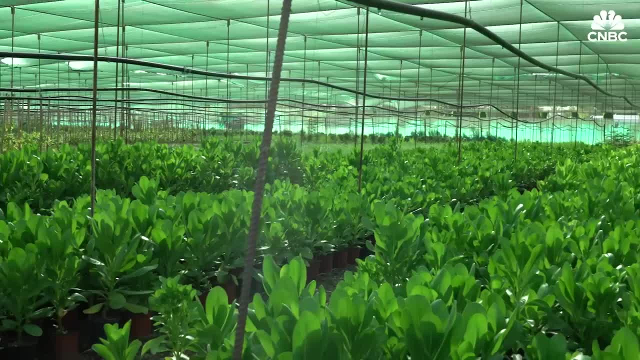 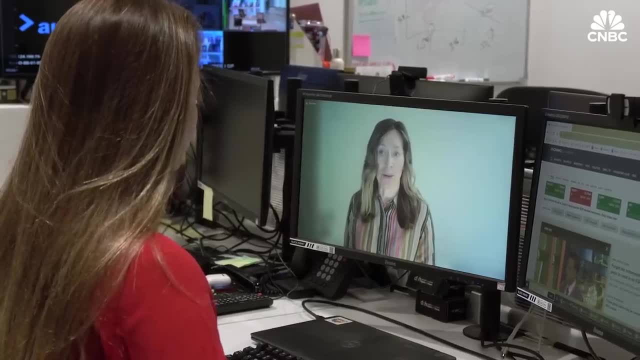 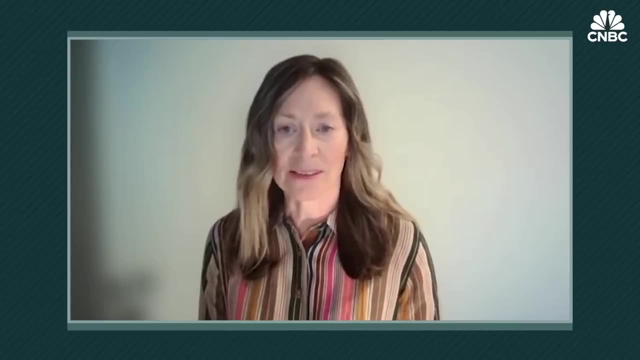 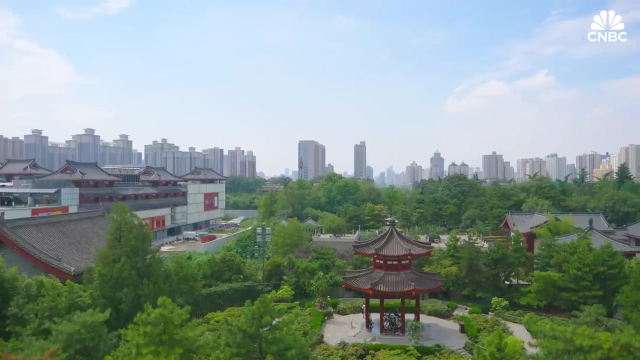 green economy. Plants are a miracle worker in terms of pulling carbon dioxide. The UEE is not alone in its quest to green the desert. Other countries like China have followed the same path, as seen in a desert called Kibuchi in the country's Inner Mongolia Autonomous Region. 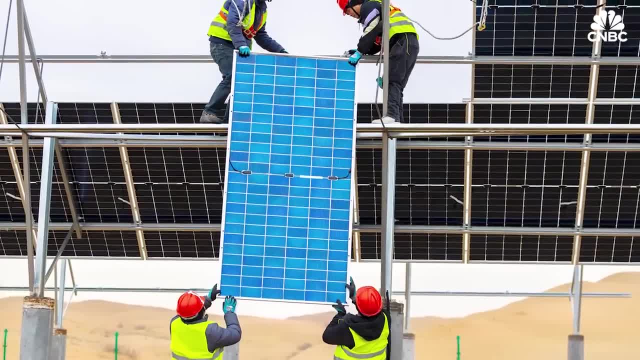 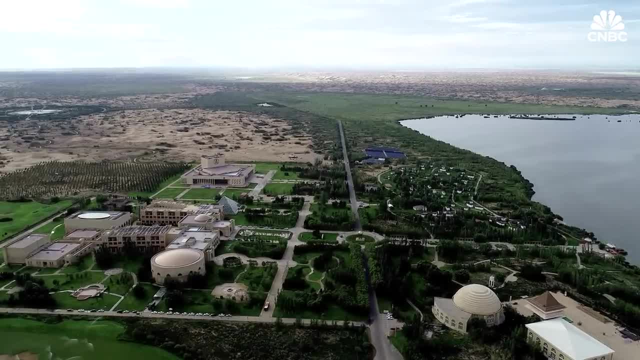 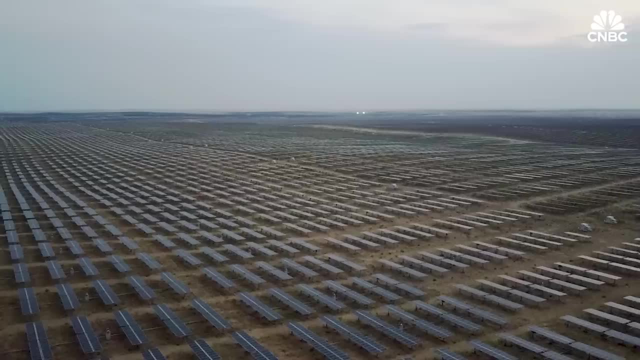 In 1988, a Chinese company partnered with the Beijing government to build solar farms and other renewables. Three decades later and one-third of Kibuchi is green, preventing dunes from enroaching on farms. The United Nations Environment Program estimated the Kibuchi project cost $1.8 billion over 50 years. 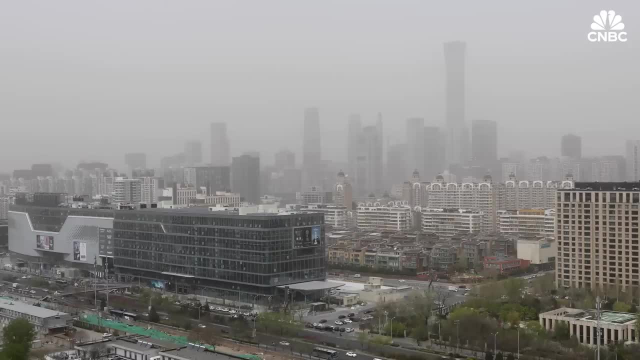 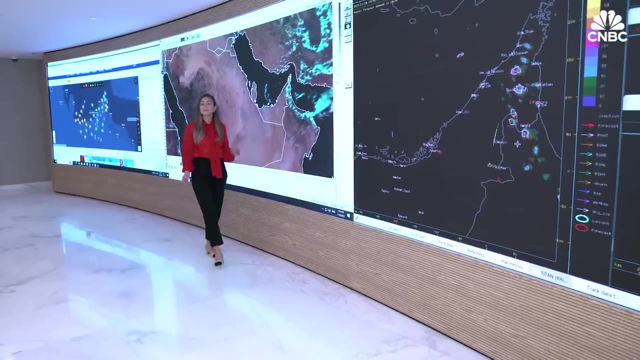 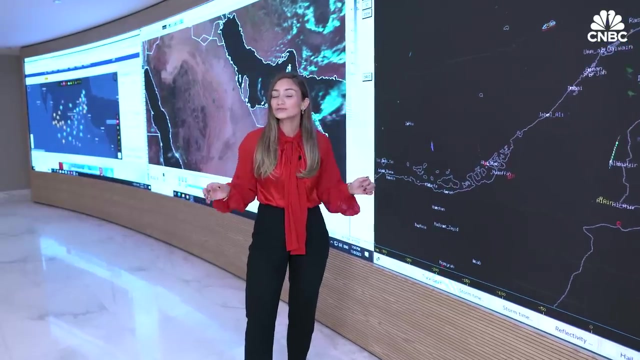 Beijing is a proponent of cloud seeding technology. They used it to manipulate weather, to protect farming areas and to guarantee clear skies for key events. The UEE performs around 1,000 hours of cloud seeding to enhance rainfall in just one year, and it's all controlled in this building, the National Center of Meteorology in. 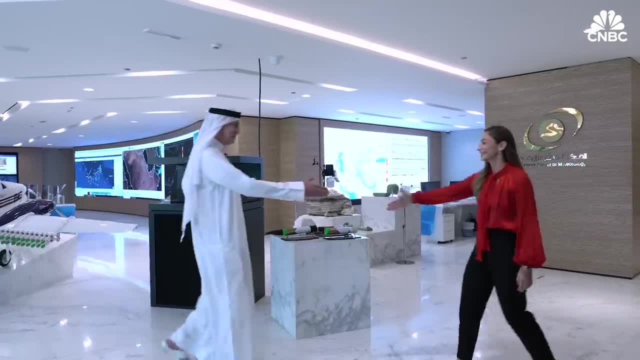 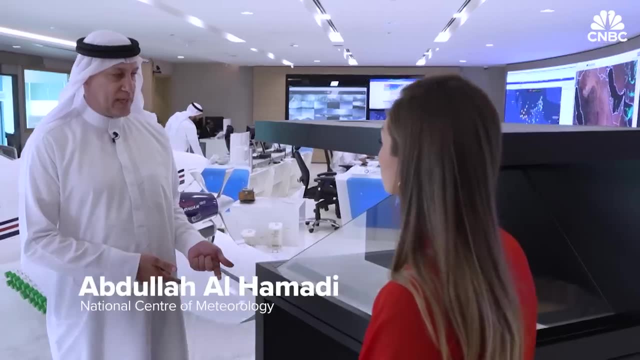 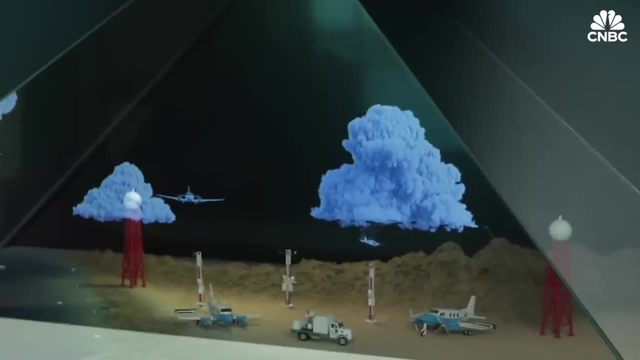 Abu Dhabi where they track the whole process. We met with a cloud seeding expert to explain how the seeding process works. We wait for the forecast. when we have a good chance for a cloud, We send the aircraft to that location, go under the cloud in the first stage of the cloud there is. 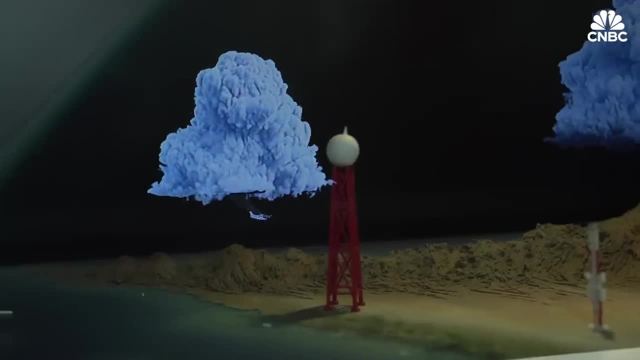 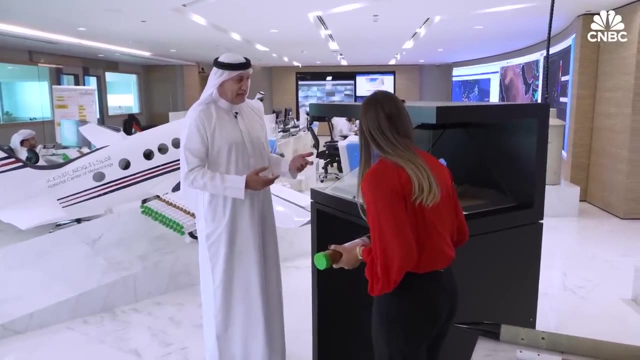 good updraft. at that time start to release all the salt And with the good updraft the seeding is done. The good updraft, of course. it will go inside the cloud and start to condensate and the droplets will become bigger and start to rain. 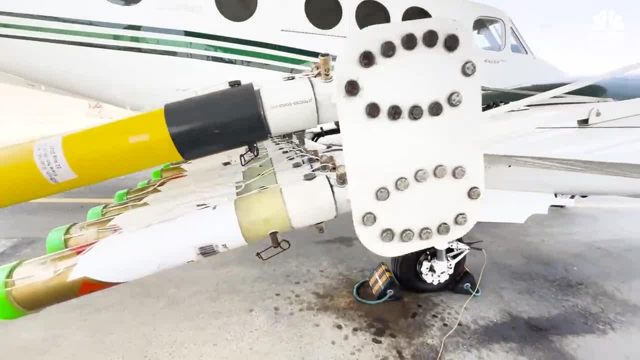 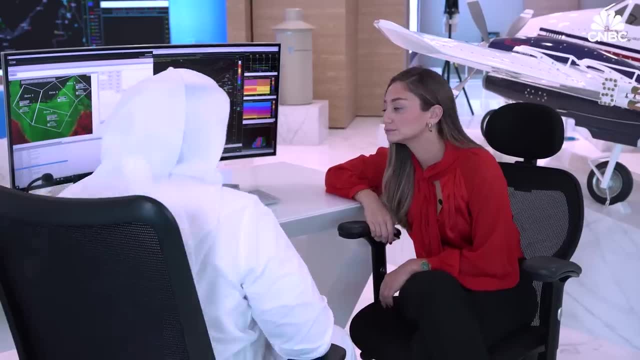 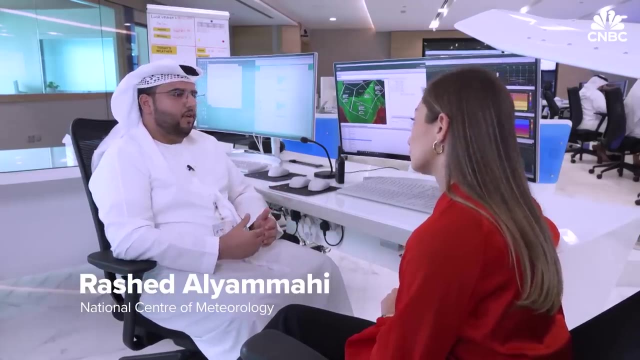 The center manufactures a salt substance that helps enhance rainfall. They put them in what they call flares- Operation 219.. We also spoke to one of the weather forecasters. He explains how the operations work. We align our pilots to be on the airports and tell them when to be at the airport.